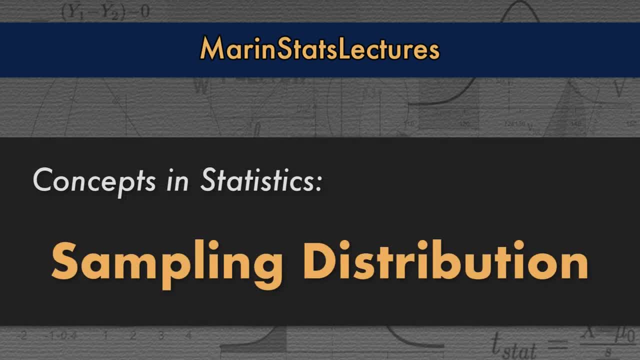 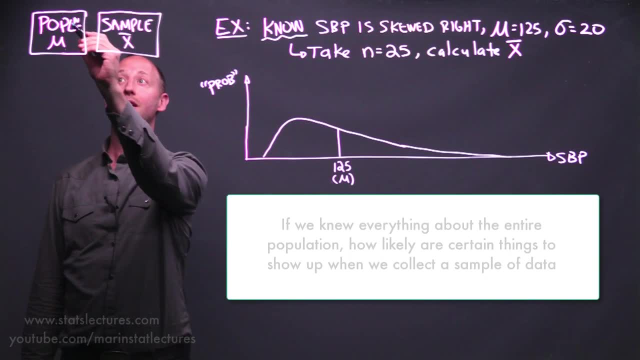 In this video we're going to build up the concept of a sampling distribution and, specifically, we're going to talk about the sampling distribution of the mean. This is going to help us to understand if we knew the truth for the entire population. how likely are certain things to show up when we collect a sample of data? 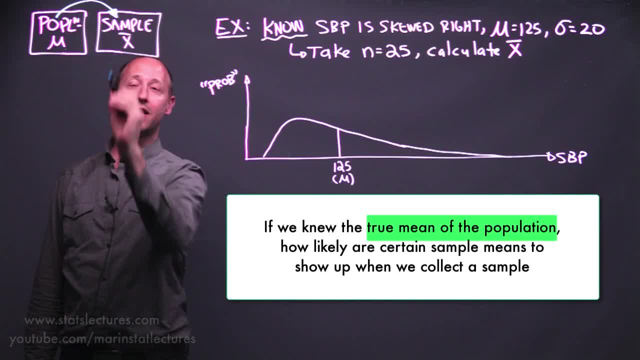 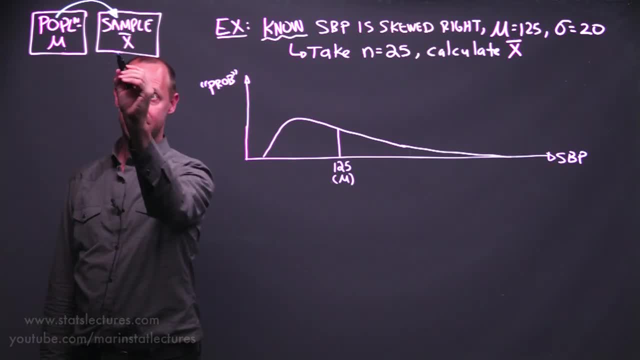 Specifically, if we knew the true mean in the population, how likely are certain sample means to show up when we collect some data? Building this understanding is going to help us to do statistical inference, where we take our sample and try and make statements about the population. 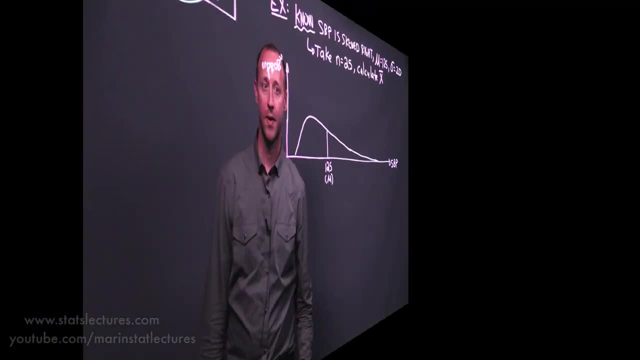 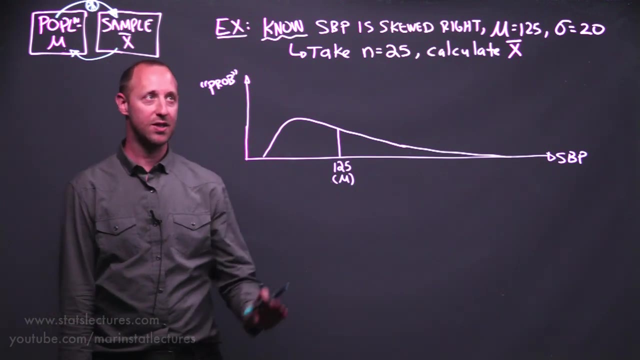 So first let's build up these concepts here. So to do this, we're going to live in the pretend world for a little bit and we're going to suppose that we know at the population level systolic blood pressure has a distribution that's skewed to the right. We know the true mean is 125,. 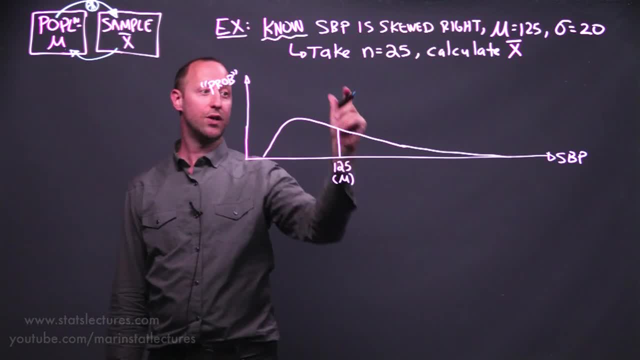 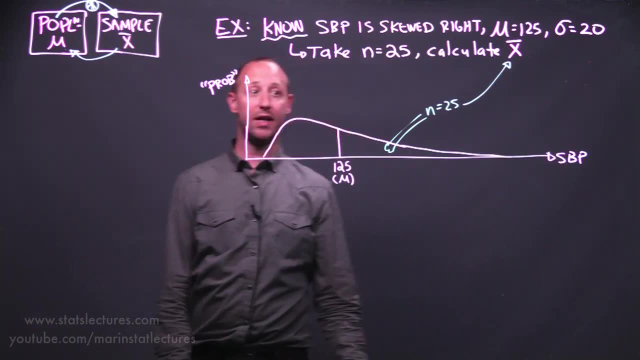 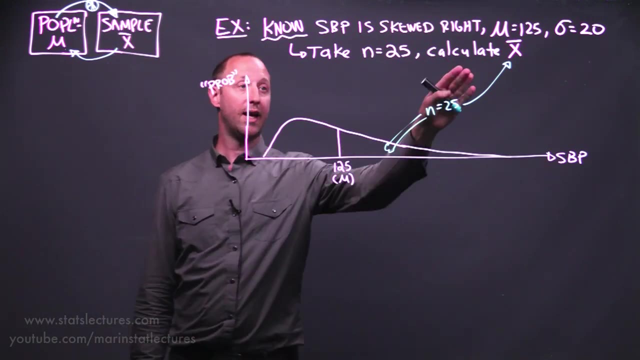 the true standard deviation is 20, and we're going to reach into this population here. We're going to take a sample of 25 observations and we're going to calculate a sample mean. Now, in reality, we're just going to take one sample of size 25 and get one sample mean. 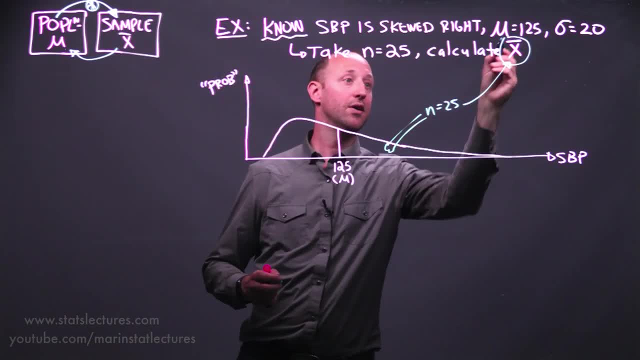 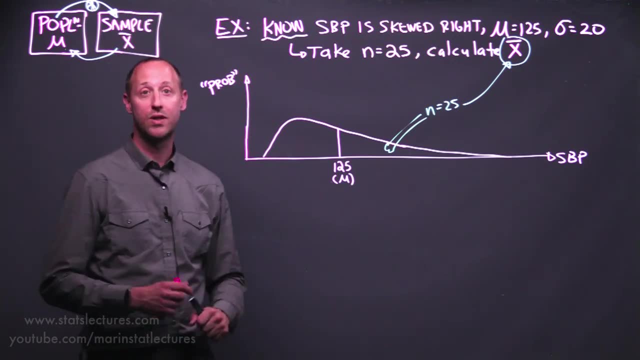 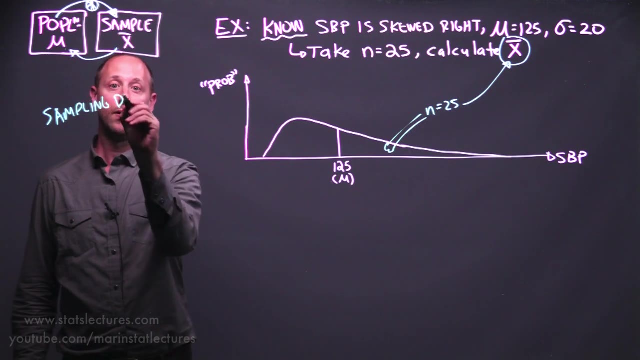 but we learn to think of this sample mean here as one of many we could have got. We could have ended up with a slightly different set of data which would have given us a different estimate. This builds the idea of a sampling distribution, And the sampling distribution is the theoretical set of. 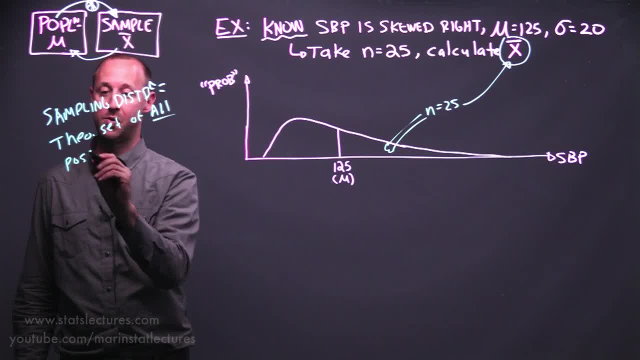 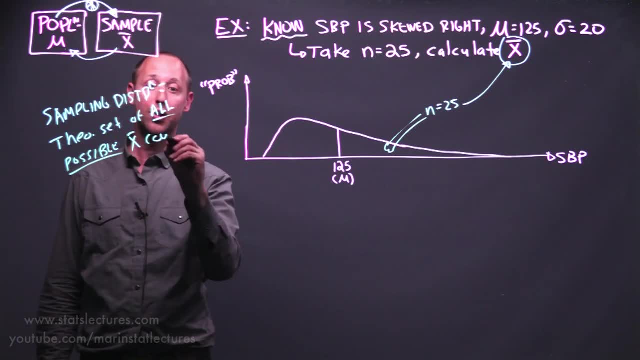 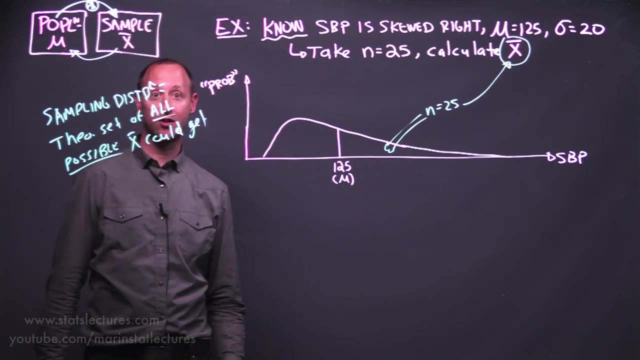 all possible estimates or sample means. we could get Okay again. In reality, we only end up with one, but we think of it as one of many. we could have Get Okay again. In reality, we only end up with one, but we think of it as one of many we could have gotten. 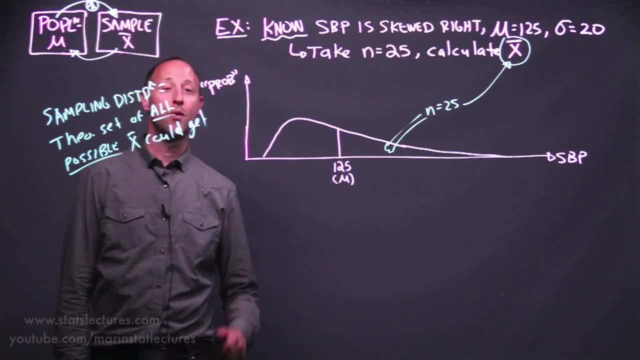 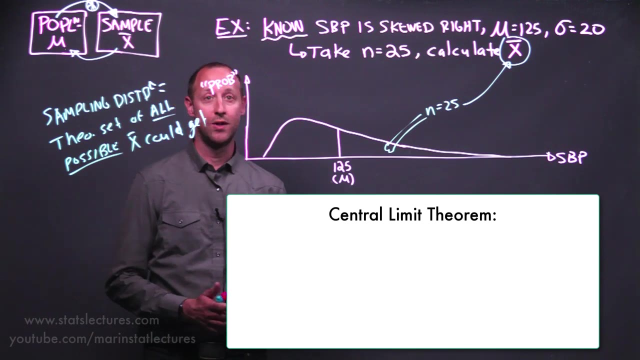 have possibly got. So to build up this concept, we're going to imagine taking samples of size 25 over and over again from this population and looking at the distribution or the set of all the possible estimates we could have got. So we have this idea of the central limit theorem, which 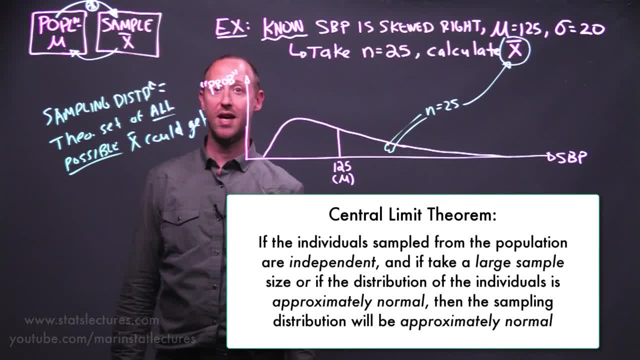 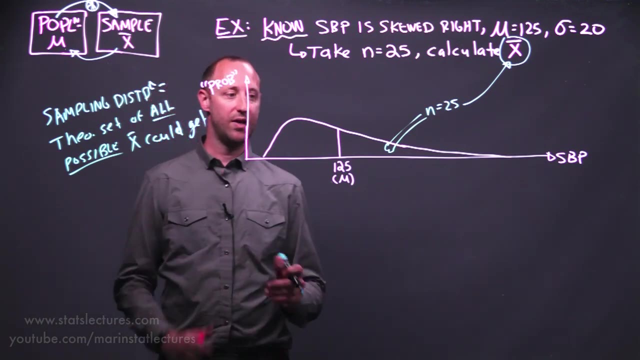 basically tells us, if the individuals we take, that we sample from the population, are independent and we take either a large sample size or the distribution of the individuals is approximately normal, then the sampling distribution, this theoretical set of all the estimates we could have ended up with, will be approximately normal. So we can think of when we collect our sample of. 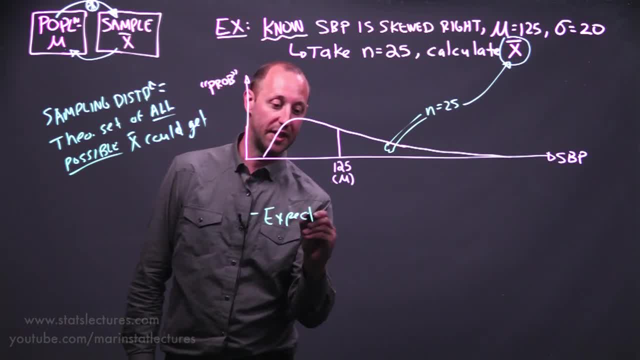 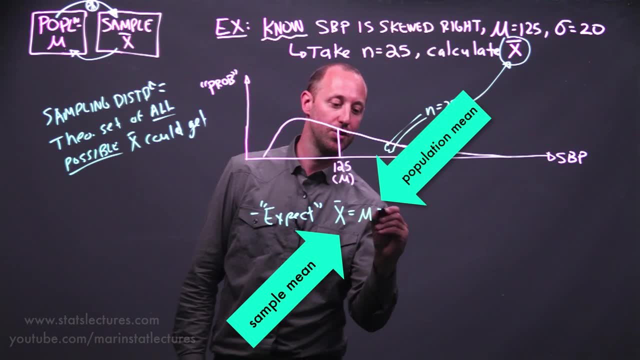 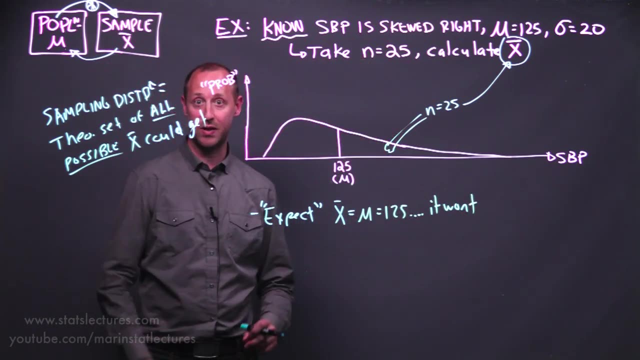 25 observations. we expect and expect in the statistical sense. we expect that our sample mean and expect that our sample is going to be equal to the true mean of 125, but we know that it won't. so again, the statistical meaning of expect on average if we took repeated samples over and over the mean of all the sample. 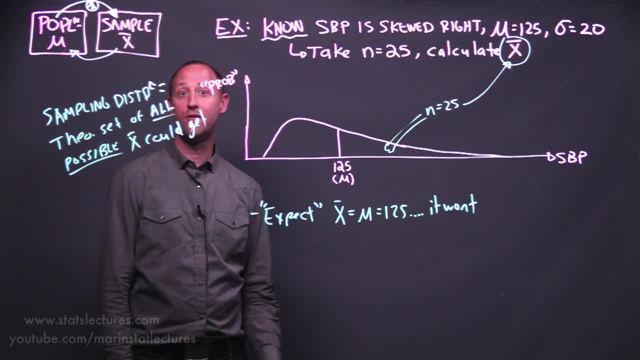 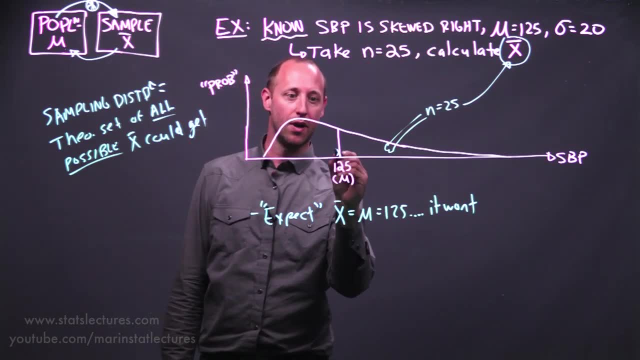 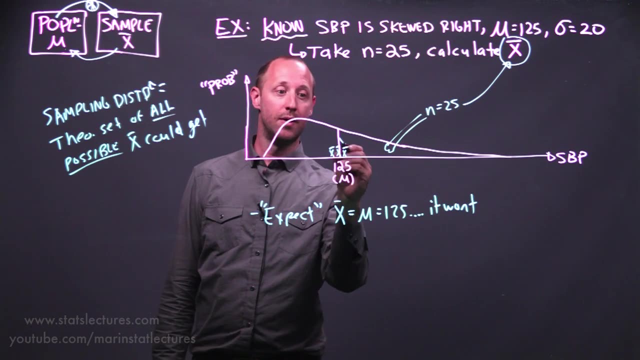 means would be 125.. similar to the idea that if you toss a coin 100 times, you expect to get 50 heads. chances are you won't. so we expect our sample mean to be equal to the true mean. we know that it won't be. we might get something a little bit above or a little bit below, but if we took 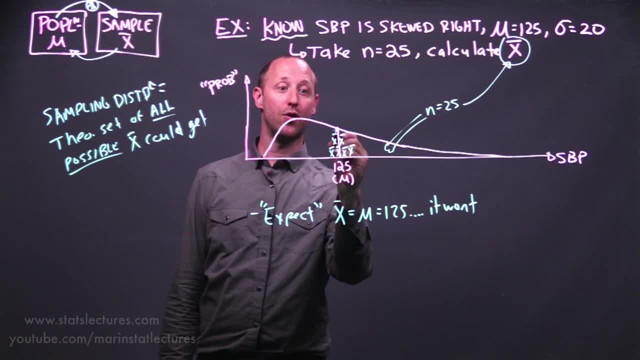 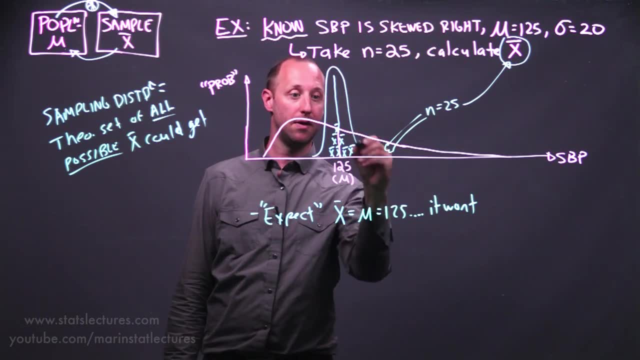 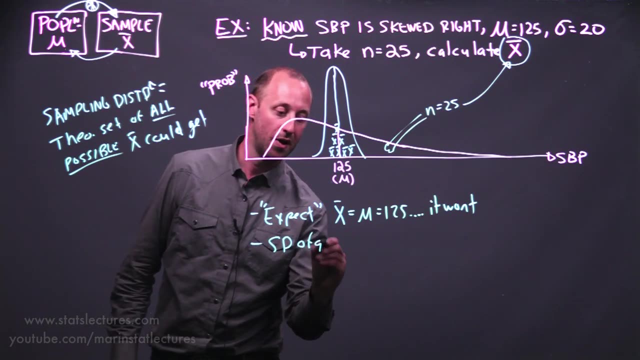 samples over and over again and calculated sample means over and over again and looked at the distribution. okay, our histogram of all these. it would be approximately bell-shaped, centered around the true mean. we can think of the standard deviation of all these possible sample meanings that we can get. we call that the standard deviation of x bar. 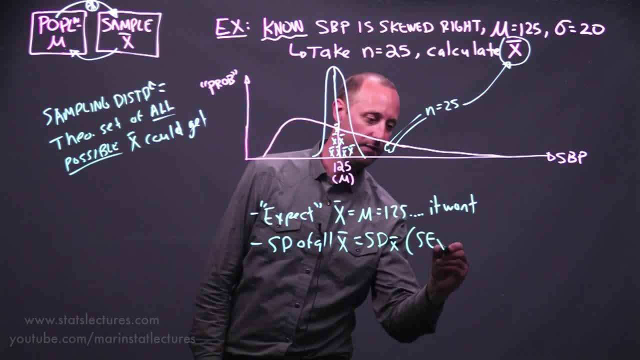 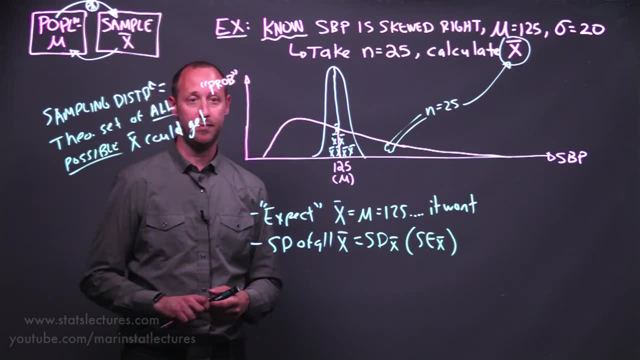 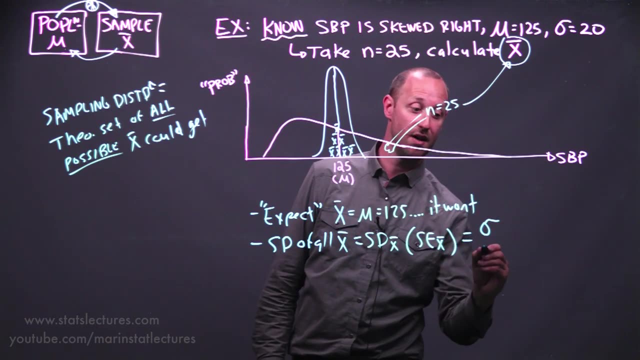 or often once we move into dealing with only samples of data. we're going to call it the standard error of the mean. standard deviation of the mean. standard error of the mean. exact same concept. without any justification for the moment. this comes out to be the standard deviation of the. 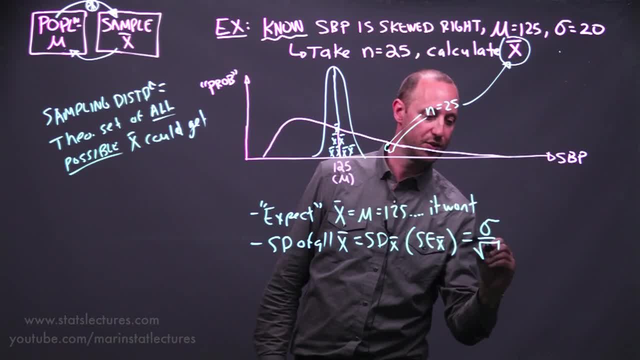 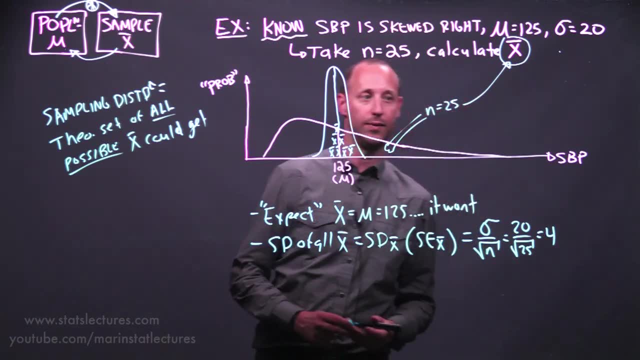 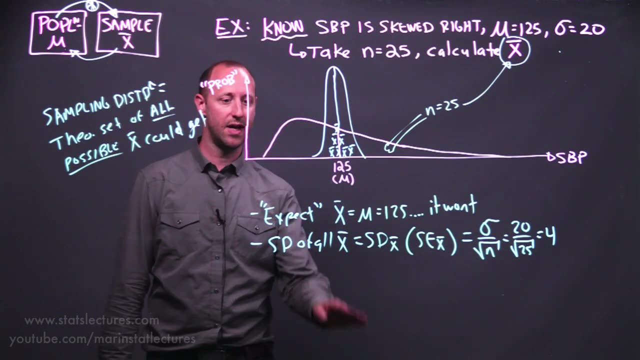 individual observations divided by the square root of the sample size. so here 20 over square root of 25, which equals 4.. okay, again later we can talk about mathematically how do we get ourselves there. but what this standard error tells us is that while we expect our sample mean to be equal to the true mean of 125, we know that. 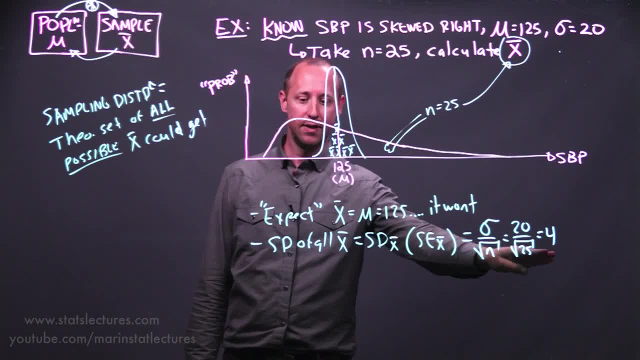 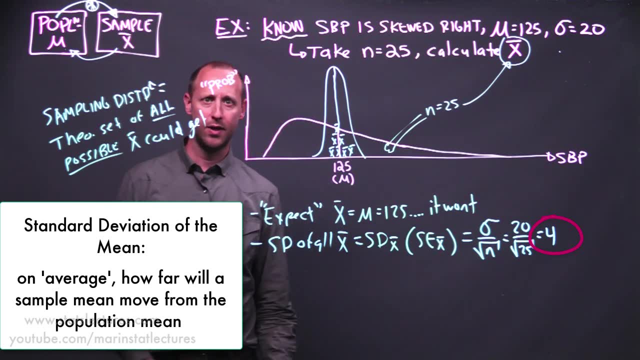 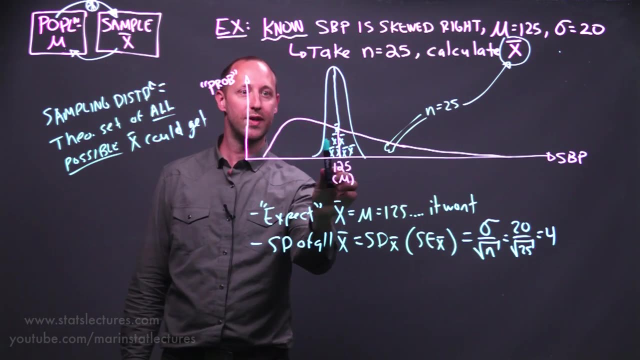 it won't. it's going to vary a bit above or below, but this standard deviation of the mean gives us an idea of, on average, how far will our estimate move from the true value. so, on average, our sample mean is going to move about 4 units from that true mean. we also know that it's going to be normally. 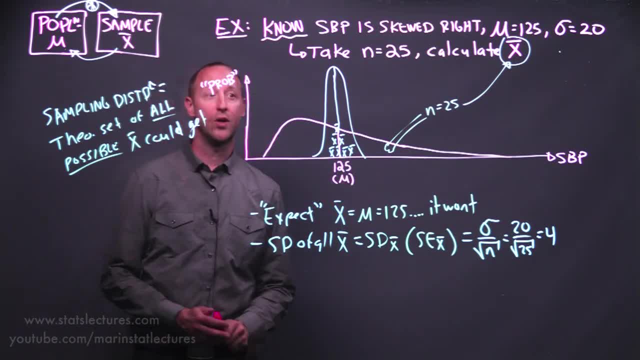 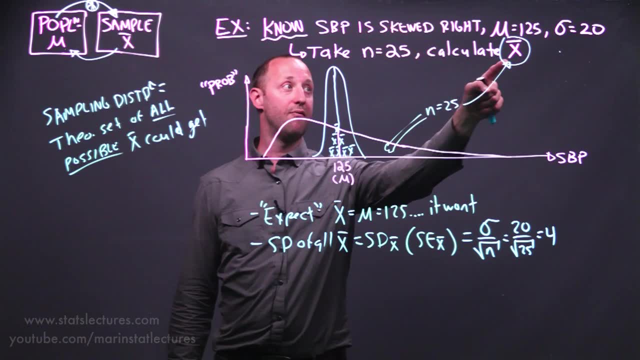 or symmetrically distributed around the true mean. so, again, to recap some of these ideas, we're going to reach into the population. we're going to select 25 individuals and for them we're going to calculate a sample mean. okay, we're only going to do this once, but we can think of it as one of many estimates. 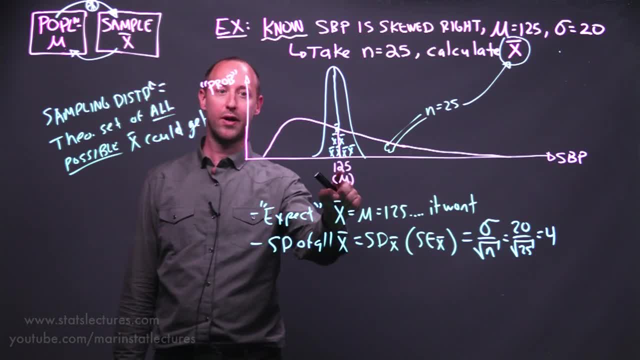 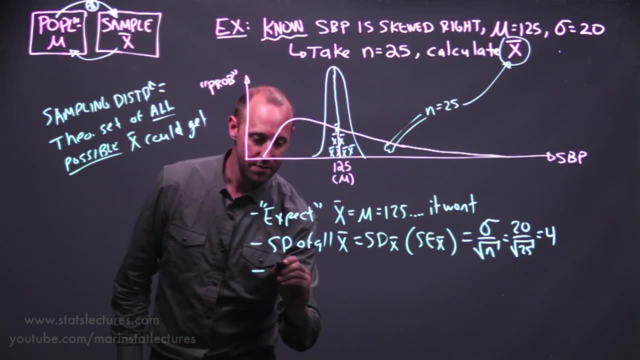 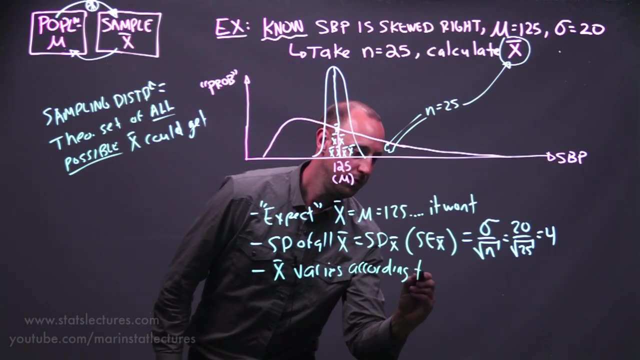 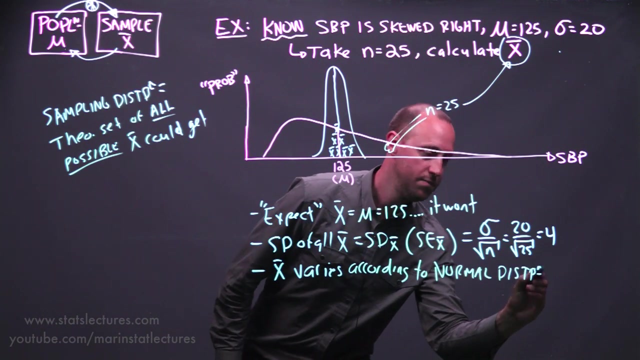 we could have possibly got. we're going to expect our estimate to be equal to the true value. we know that it won't be right. it might vary a bit above or a bit below, but the sample mean varies according to a normal distribution, meaning it's normally or symmetrically distributed around the true value. okay, and again the standard. 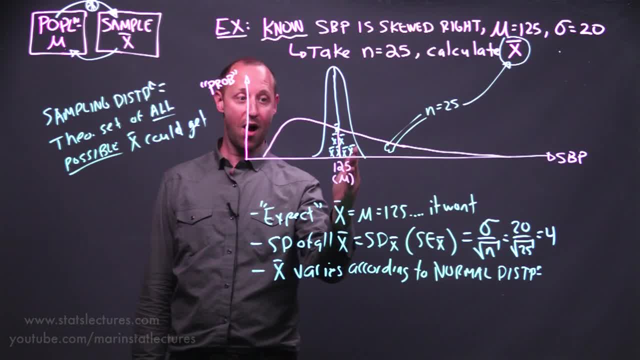 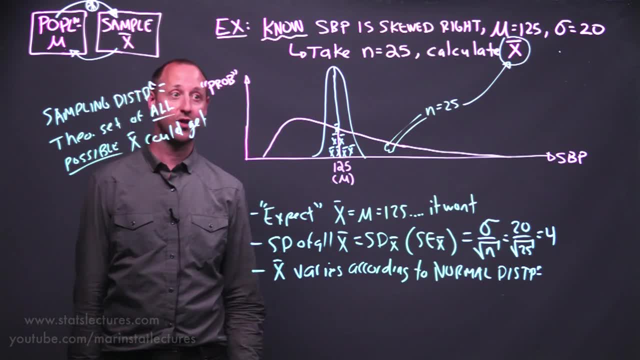 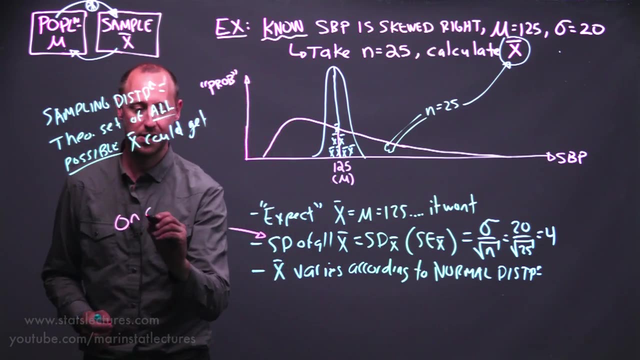 error gives us an idea of, on average, how far will our estimate move from the true value. another way to think of this: the standard deviation of the mean, or what we're going to start to call the standard error. let's write it here down, because this is important. This gives us an idea of, on average, how far 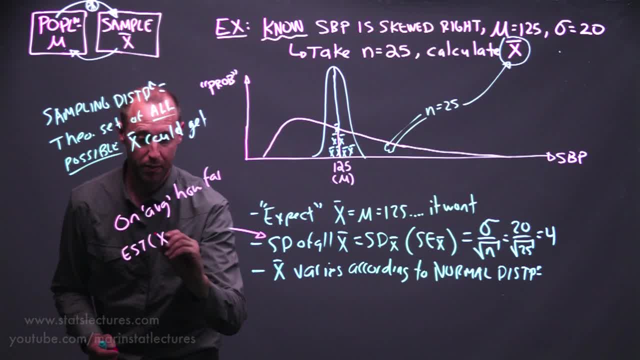 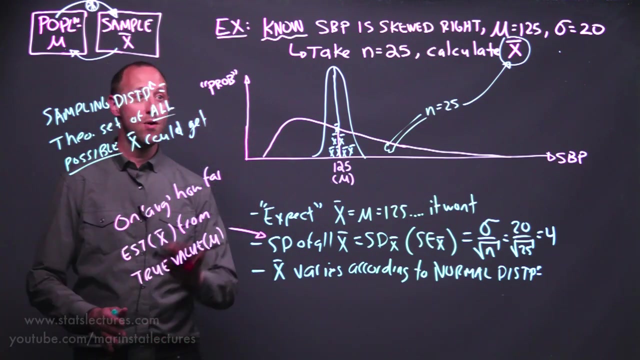 will our estimate, the sample mean, move or deviate from the true value? mu? If we reverse the way we're thinking about it, we can think of it. this tells us, on average, how close will our estimate be to the true value. Okay, so again. well, 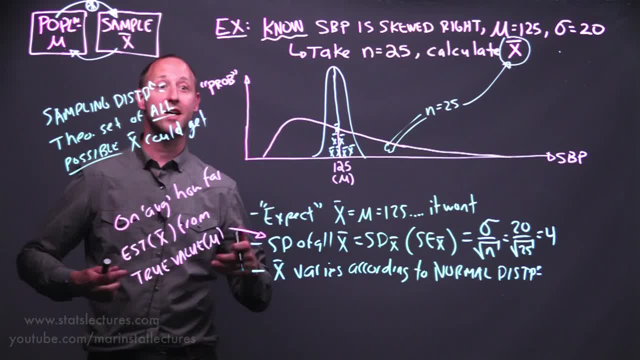 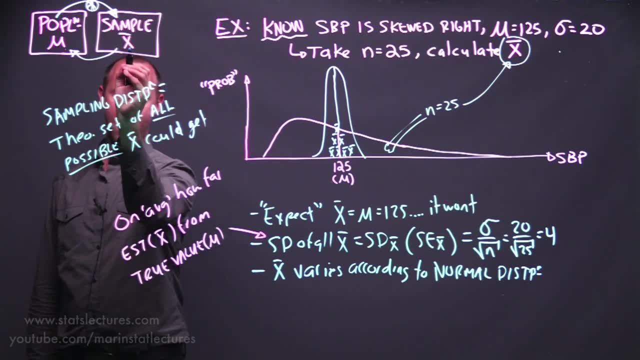 right now we're in this pretend world. we can see getting this idea of a standard deviation of the mean or standard error is going to give us an idea on average how far or how close is our estimate to the true mean. We're going to use this.